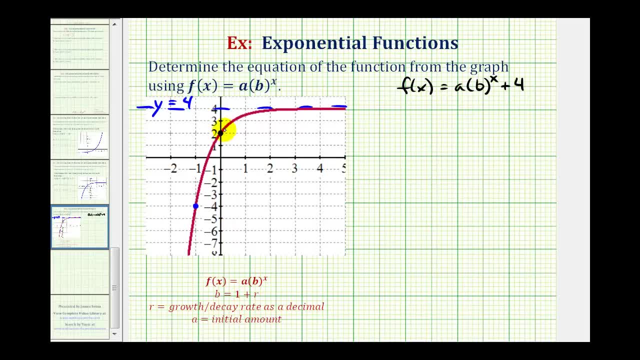 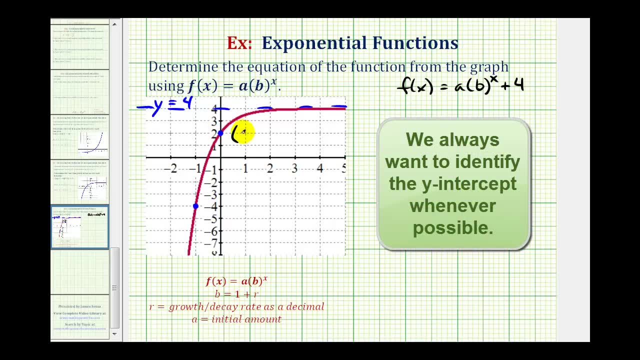 then we can determine the values of a and b by identifying two points on the function. that will give us two function values. So notice how this point here, or the y-intercept, is zero, comma two, and this point here is the point negative one, negative four. 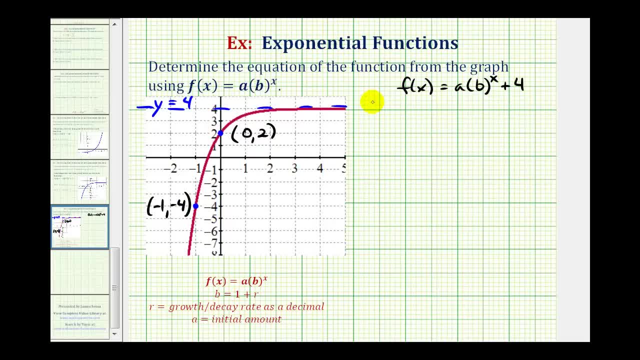 which means, if the function contains the point zero, two, f of zero must equal two, and if the function contains the point negative one negative four, then f of negative one must equal negative four. Now that we know, f of zero equals two. 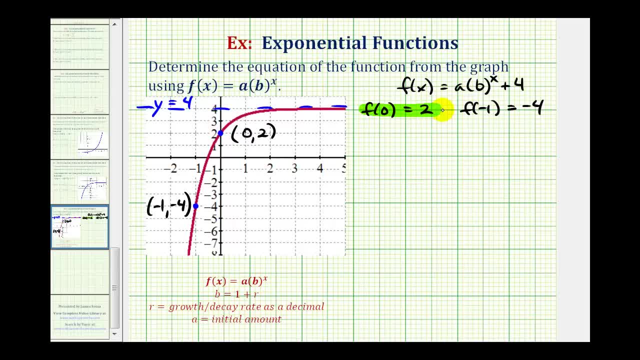 we should be able to use this to determine the value of a, and then we can use the second function value to determine the value of b. So if f of zero equals two, we'll replace x with zero, so we would have a times b to the zero plus four. 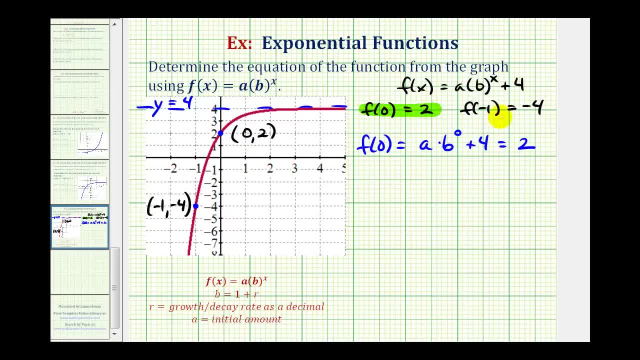 must equal positive two. Well, b to the zero is equal to one, so we have a plus four equals two. subtract four on both sides, So we have a equals negative two. So now we know that f of x must equal negative two times b to the power of x. 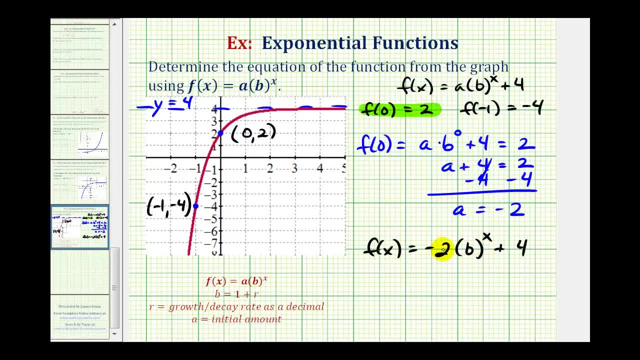 plus four. Notice how a is negative, which is what we thought, because it does look like this is exponential decay reflected across the x-axis. So now we'll use this form of our function and our second function value to determine the value of b. 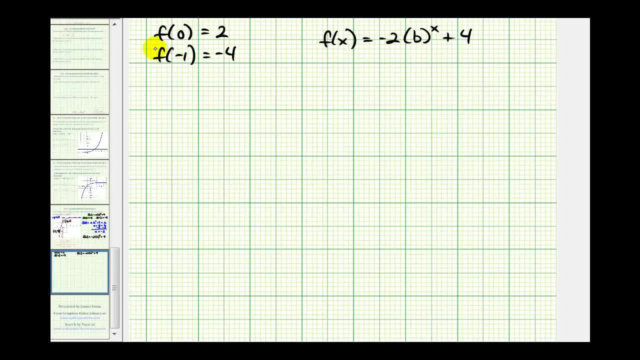 And let's go ahead and do that on the next slide. So we were able to use f of zero equals two to determine the value of a, And now we'll use f of negative one equals negative four to determine the value of b. So f of negative one. 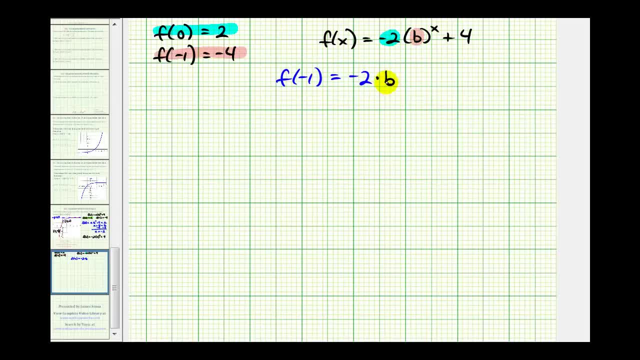 is going to be equal to negative two times b to the negative one, plus four, which must equal a negative four. So the first step, let's go ahead and subtract four on both sides, So we have negative two. b to the negative one equals negative eight. Now I'm going to make this into a fraction. 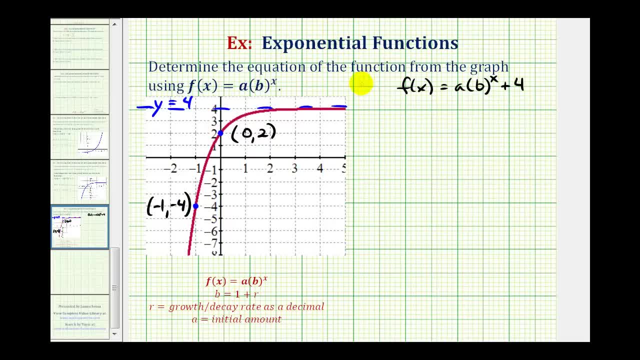 which means, if the function contains the point zero, two f of zero must equal two, and if the function contains the point negative, one negative four. f of x equals a, Then f of negative one must equal negative four. Now that we know, f of zero equals two. 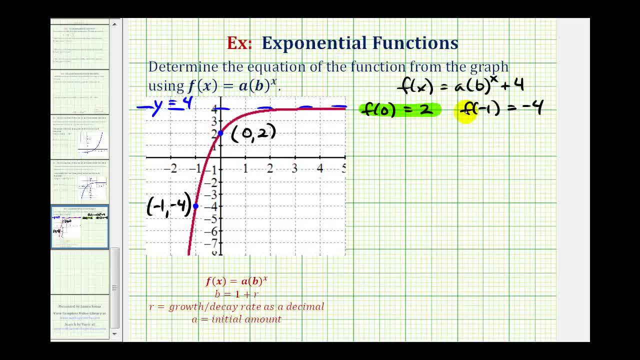 we should be able to use this to determine the value of a, and then we can use the second function value to determine the value of b. So if f of zero equals two, we'll replace x with zero, so we would have a times b to the zero plus four. 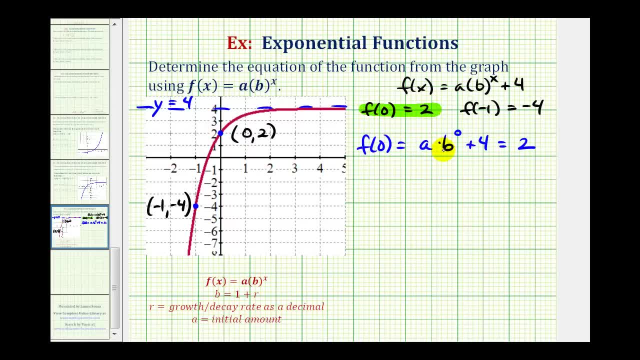 must equal positive two. Well, b to the zero is equal to one, so we have a plus four equals two. Subtract four on both sides, So we have a equals negative two. So now we know that f of x must equal negative two. 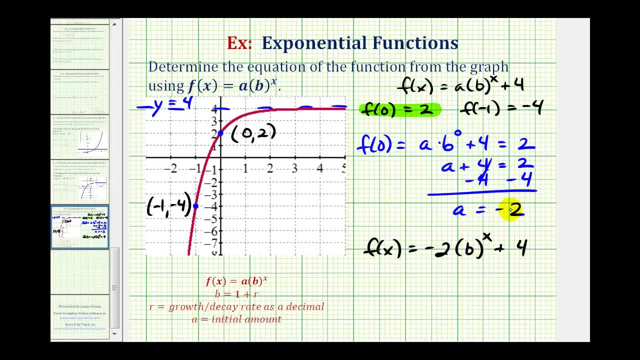 times b to the power of x plus four. Notice how a is negative, which is what we thought, because it does look like this is exponential decay reflected across the x-axis. So now we'll use this form of our function and our second function value to determine the value of b. 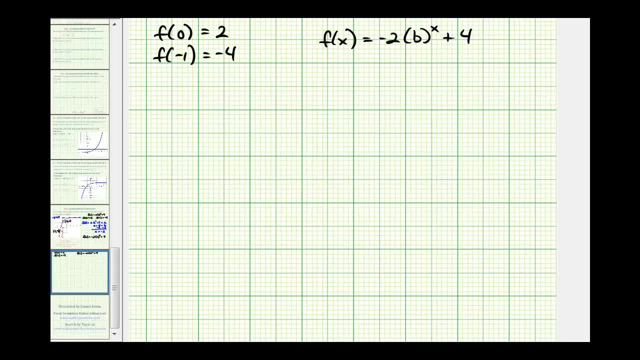 And let's go ahead and do that on the next slide. So we were able to use f of zero equals two to determine the value of a, and now we'll use f of negative one equals negative four to determine the value of b. So f of negative one is going to be equal to. 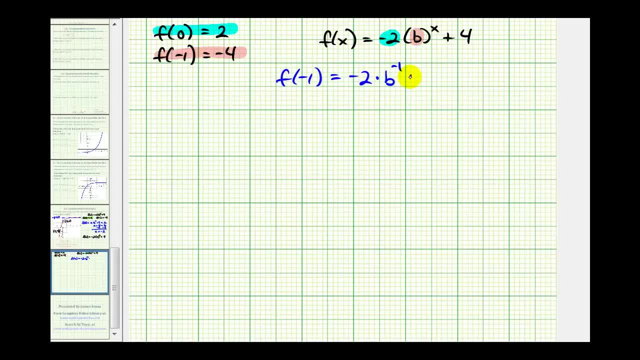 negative two times b to the negative one, plus four- which must equal it- of 4.. So the first step: let's go ahead and subtract 4 on both sides, So we have negative 2 b to the negative. 1 equals negative 8.. I'm going to make this into a. 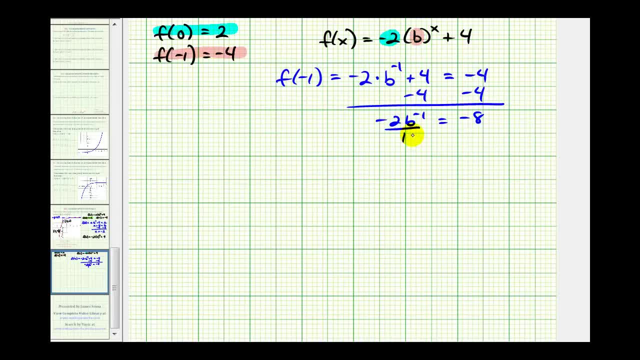 fraction. Remember, if I move the b down to the denominator, it's going to change the sign of the exponent. So we would have negative 2 over b equals negative 8.. And now we're going to multiply both sides of the equation by b. This is b. 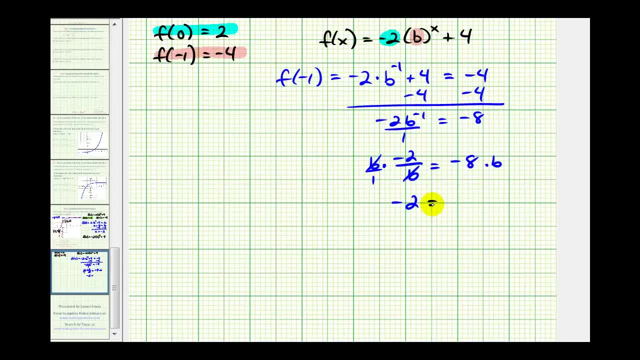 over 1, so the b's simplify out. We have negative 2 equals negative 8 b. Now we can divide both sides by negative 8.. So we have b equals- this simplifies- to positive 1. fourth, So now that we have b, we have our function. Our function is f.